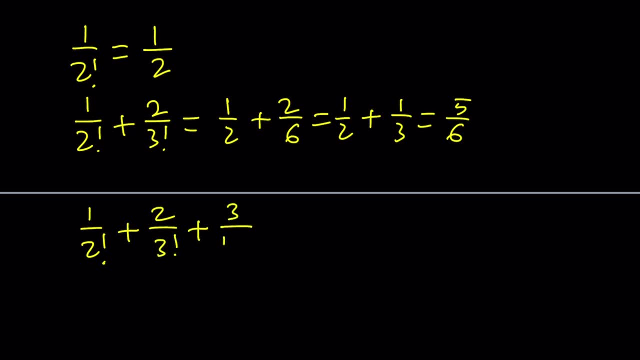 or at least we'll have an idea, And when the actual result comes up it shouldn't be a huge surprise. So now I'm basically adding 3 over 4 factorial, which is 1 eighth to this, So it's kind of like 5 over 6, which comes from here. 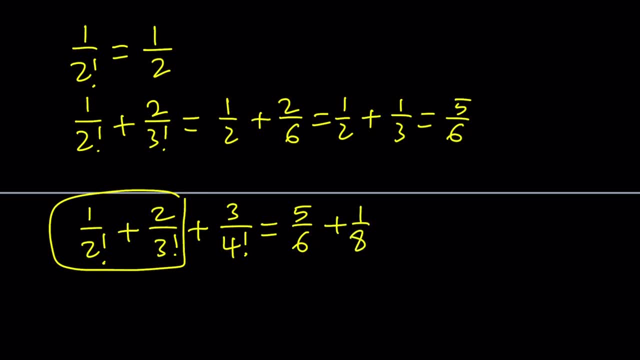 plus 1 over 8. The common denominator is 24.. So let's go ahead and multiply by 4 here and 3 here. That's going to give us 5 times 4 plus 3, which is 23 over 24.. 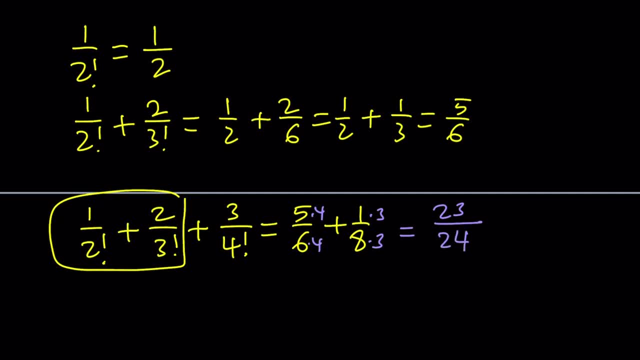 Hmm, that's kind of interesting. So what I'm seeing here is, so far, the denominator is always 1 less than the numerator, And if you're not convinced- and obviously that's not going to- there's not going to be. 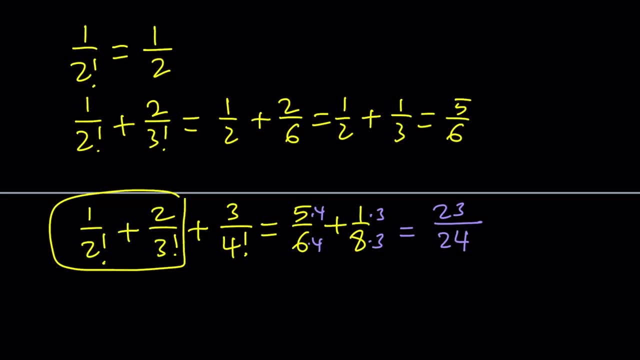 a proof by any means, but at least it should give you an idea. Okay, I'm not completely convinced, but I think there is a difference: of 1. And you can do more and more on this, But that's what I'm thinking. Okay, what about the denominators? Look at the denominators. The denominators are. 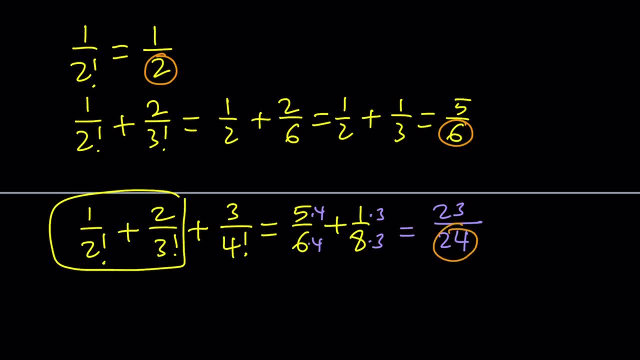 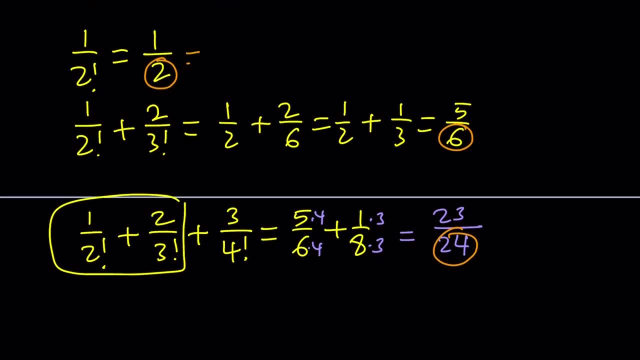 special in some sense, to 6 and 24.. What does that remind you? Well, we're looking at factorials, aren't we? So are they factorials? And the answer is yes. So this is like 1 over 2 factorial, This. 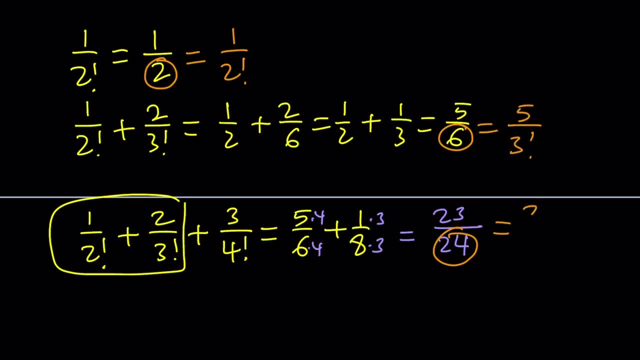 is like 5 over 3 factorial And this is like 23 over 4 factorial. Okay, great, But where does the 5 come from? Since 5 is 1 less than 6, we could also write it as follows: We can write this as: 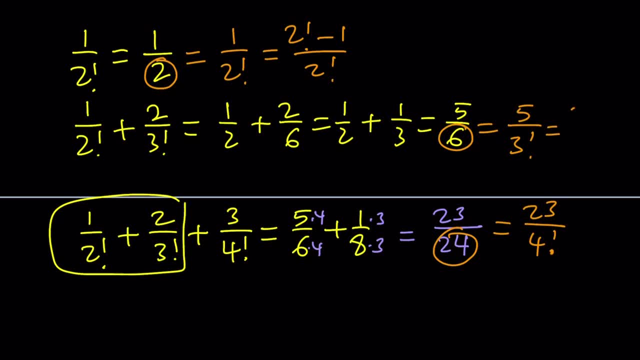 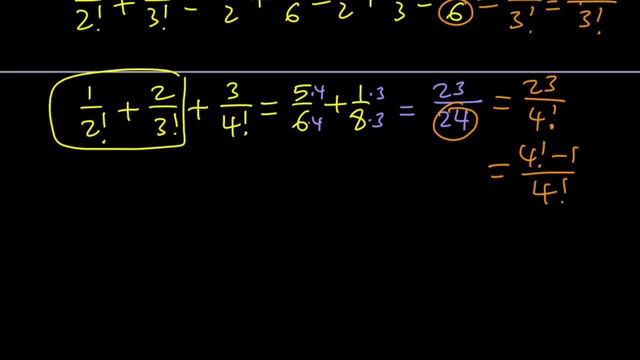 factorial minus 1 over 2 factorial And we can write this as 3 factorial minus 1 over 3 factorial And we can write this as 4 factorial minus 1 over 4 factorial And in general, if this is true in. 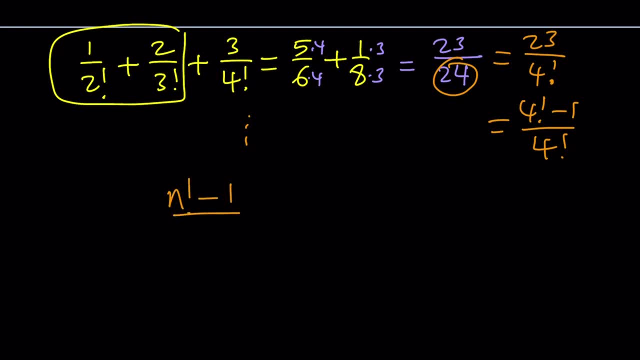 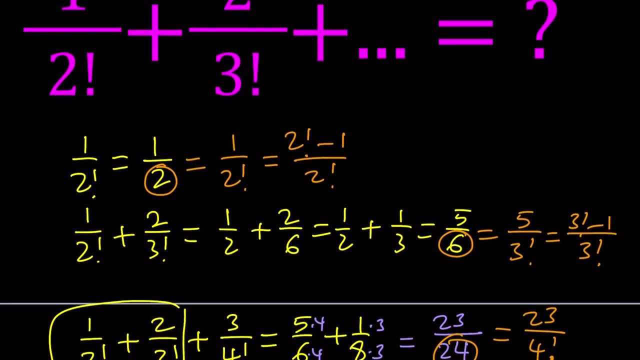 general, then it should be something like n factorial minus 1 over n factorial, And obviously this could be split up into two fractions, such as 1 minus 1 over n factorial. So that's my guess. Let's go ahead and see how this plays out. Okay, so we have. 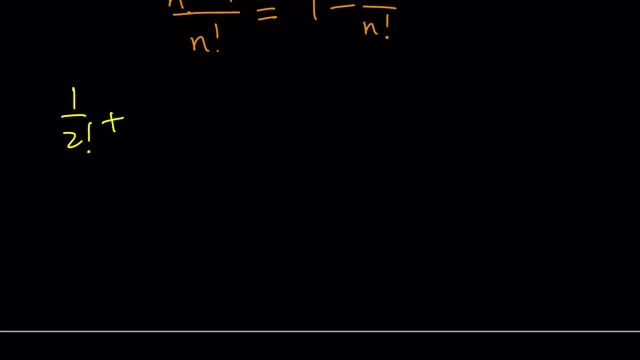 this sum: 1 over 2 factorial plus 2 over 3 factorial plus 3 over 4 factorial, and so on and so forth. There is no nth But to understand what happens. if this is an infinite, this happens to be. 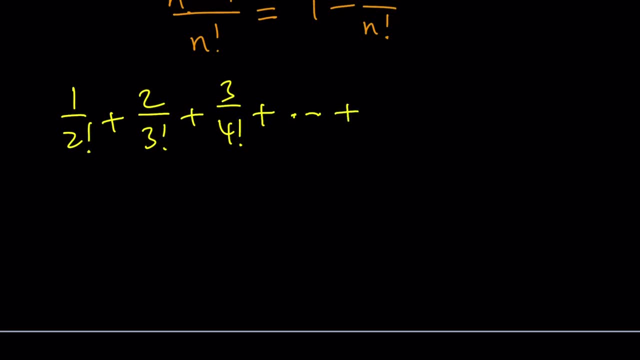 an infinite sum, then we can actually stop at some point, like, let's say, start at the nth term, that would be n over n plus 1 factorial, And then look at this sum, this partial sum, as n over n factorial plus 1 over n factorial. And this is what an infinite sum means, right, In some sense. 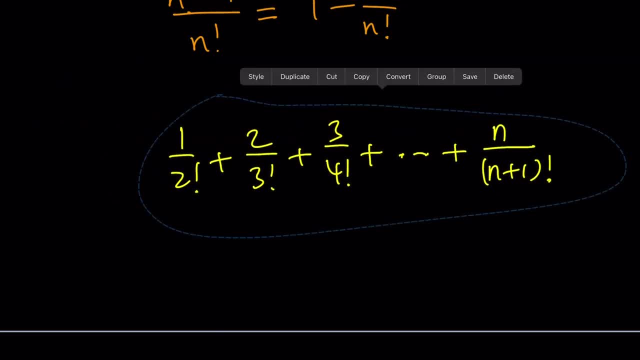 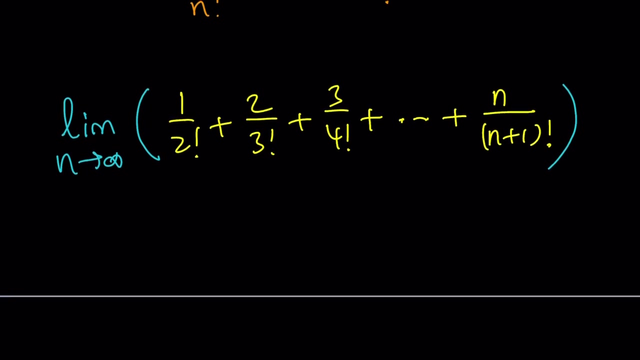 So let's go ahead and write this as a limit. So I'm going to put the limit here in the front, like this Limit as n approaches infinity of this sum. Of course we also need to talk about the convergence, so on and so forth, But when you're able to find a closed formula for this sum, 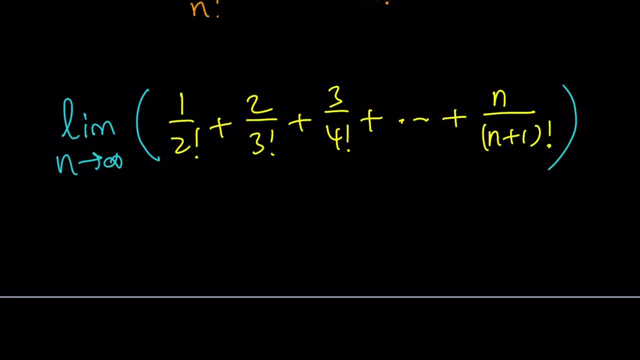 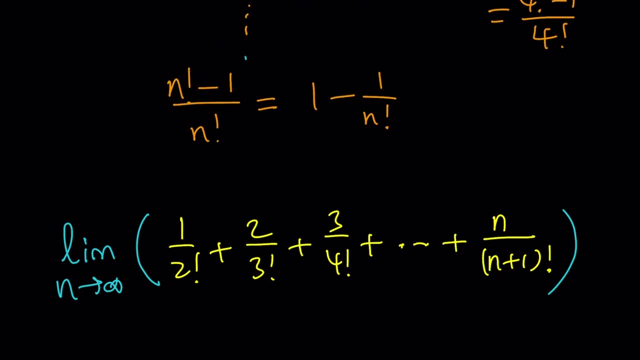 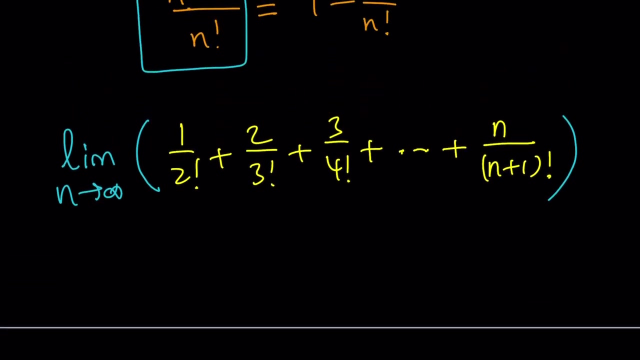 then obviously you can take the limit, And if that limit exists, then we can say it's convergent. Okay, so how do you interpret this? Well, this kind of tells me something about what I can do, Because I kind of need to break it down. Notice that 1 is 1 less than the 2, and the 2 is 1 less. 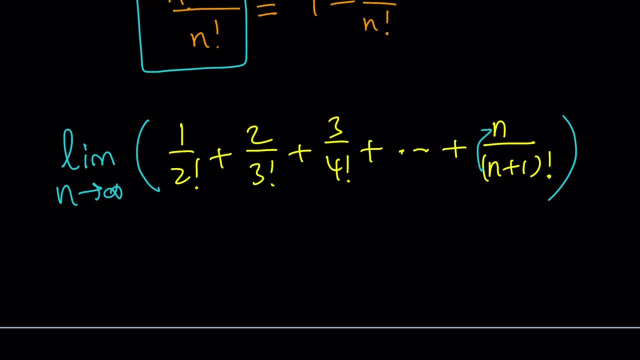 and 3 is 1 less than the 4, so on and so forth. The difference between n plus 1 and n is always 1.. Great, So can I just write the numerator as 2 minus 1 over 2 factorial then, And this one is: 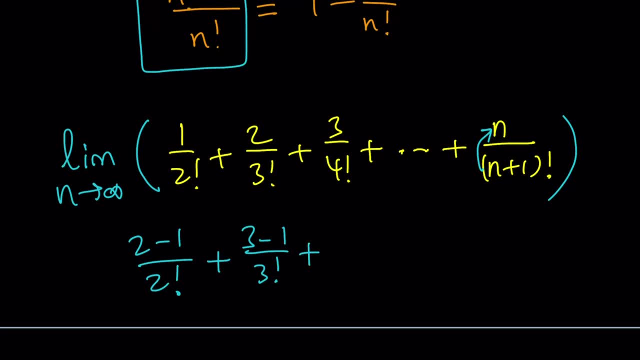 3 minus 1 over 3 factorial, and then minus 1 over 4 factorial, and all the way to the nth term, n plus 1 minus 1.. Of course I have to add 1 and subtract 1 to it, because n is a variable, and then I can go ahead and write it. 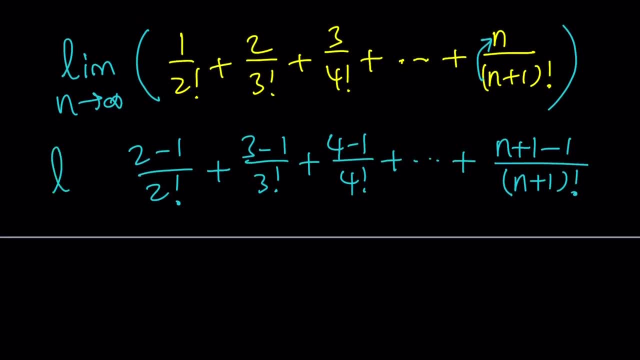 like this: Okay, now we're going to take the limit as n approaches infinity, right? So let's go ahead and take a look at what kind of sum we get from here. Now. 2 over 2 factorial is equal to what? 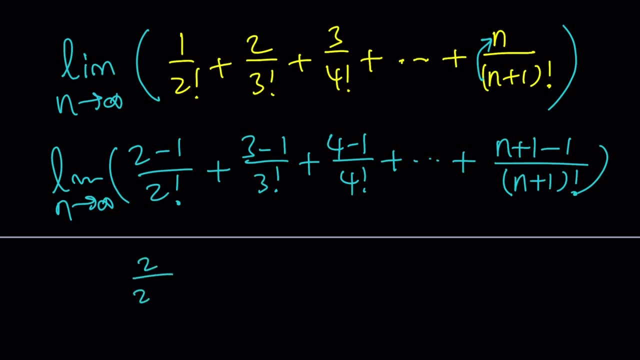 Well, 2 factorial is 2 times 1 factorial or just 1.. We can basically write this as 1 over 1 factorial, and then this gives us 3 over 3 factorial, which is 3 over 3 times 2 factorial. 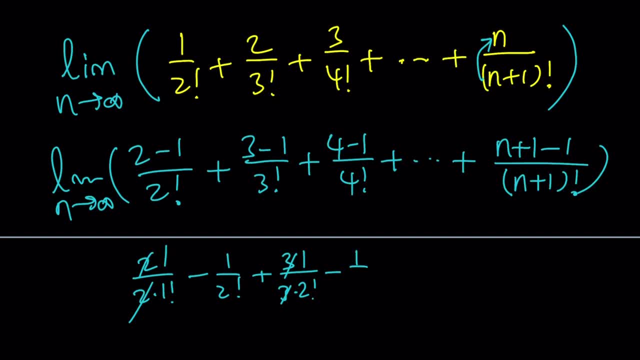 The 3's. cancel out 1 over 2 factorial minus 1 over 3 factorial and then now you've probably got the pattern: 1 over 1 factorial minus 1 over 2 factorial plus 1 over 2 factorial minus 1 over. 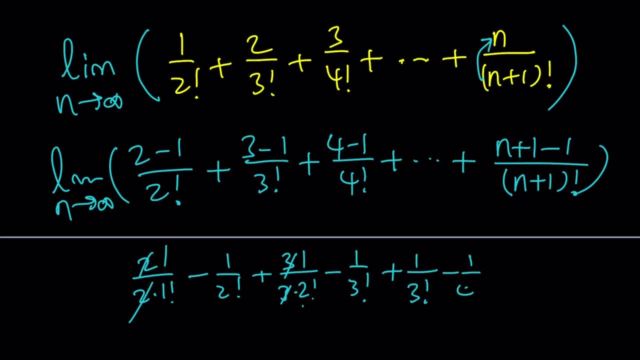 3 factorial, 1 over 3 factorial minus 1 over 4 factorial and finally, finally, we get 1 over n factorial minus 1 over n plus 1 factorial. Okay, make sense. Let's move this a little bit to the left. 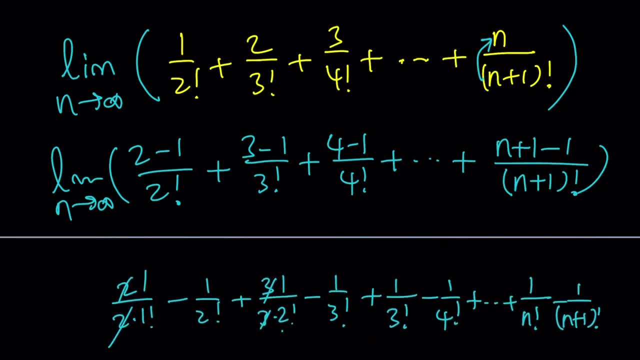 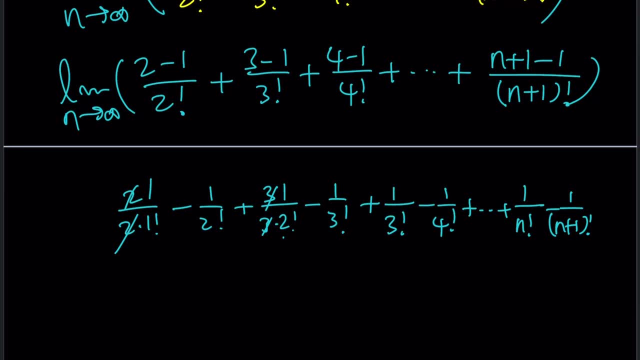 like this: Okay, so we can kind of fit it on the screen. Great, Now again, this is a limit, so let's go ahead and write it as a limit. So we're going to put the limit here as n approaches. 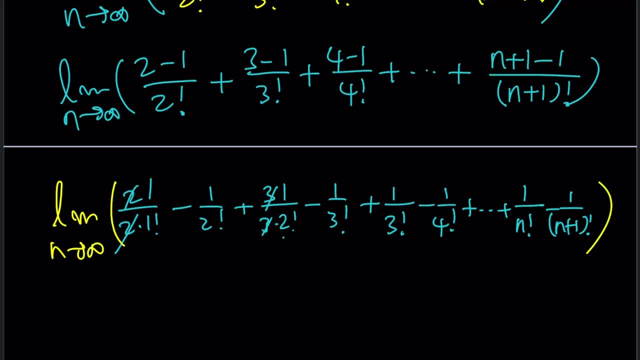 infinity. Now what we're going to do with this limit is a lot of things are going to cancel out. For example, 1 over 2 factorial is negative and positive. This is negative and positive, negative and positive, so on and so forth. Pretty much everything, except for the last term and the first. 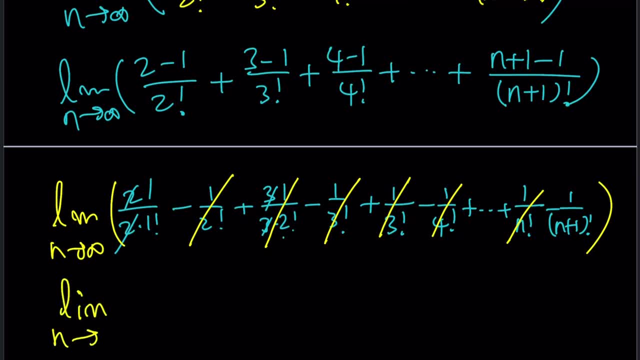 term are going to cancel out. So this is going to give us limit. as n approaches infinity of 1 over 1, factorial can just be written as 1 minus 1 over n plus 1 factorial. Obviously, n plus 1 factorial is just going to grow much faster than n, right? So as n approaches infinity, 1 over n. 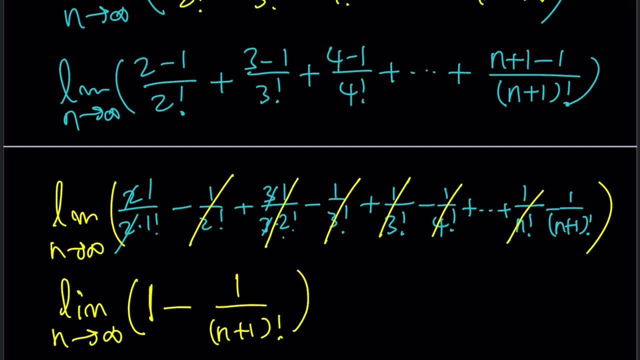 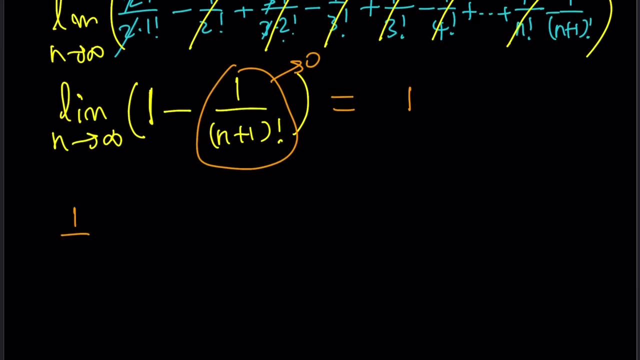 plus 1 factorial is going to approach 1 over infinity, which is 0.. So this is going to approach 0, right, And our limit is going to be 1 as n approaches infinity. What is that supposed to mean? It means that this sum that we were talking about- 1 over 2 factorial, plus 2 over 3 factorial. 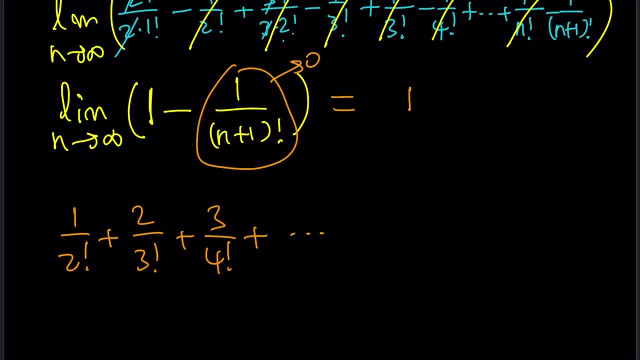 plus 3 over 4 factorial Happens to equal 1 at infinity. It's just a limit, So you can kind of talk about this for a long time, but that's not the purpose, Anyways. so we were able to evaluate this. 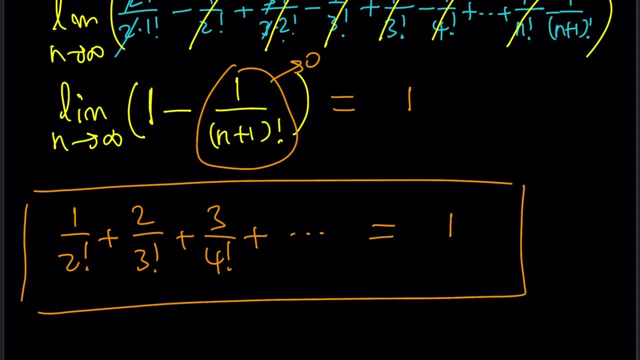 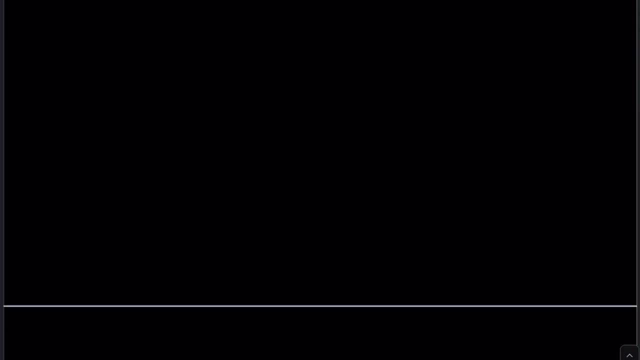 infinite sum and that happens to be 1.. Why does it converge? Because this limit exists, therefore it is convergent. Let's go ahead and take a look at some results from Wolfram Malfoy, and we're just going to finish up. So the input interpretation is like that, And then now we're going to take a.